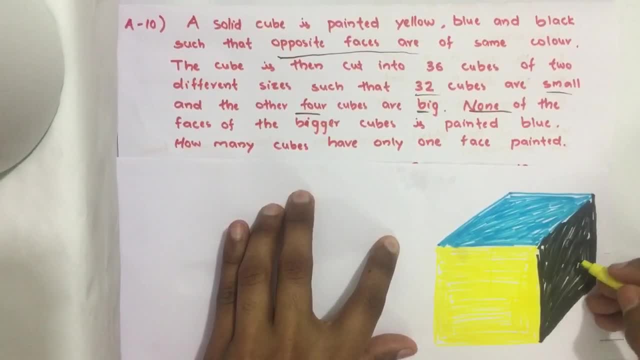 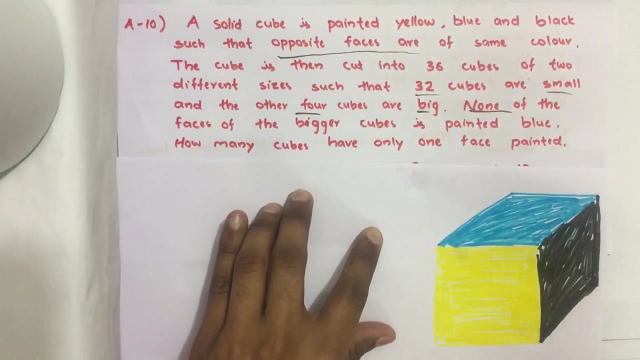 Here it is blue in bottom, it is blue. This side it is black. opposite to this it is black. And this big cube we are going to cut into 36 smaller cubes and they are also in two different sizes: 32 small cubes and four some bigger cubes, cubes. 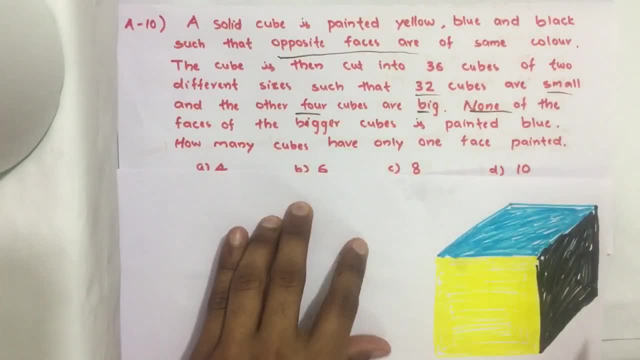 And none of the faces of the bigger cubes is painted blue. That means the cubes, the bigger cubes, which are cut from this should not have a. you know it should not change. So we are going to share any edge with this blue face. similarly in bottom. 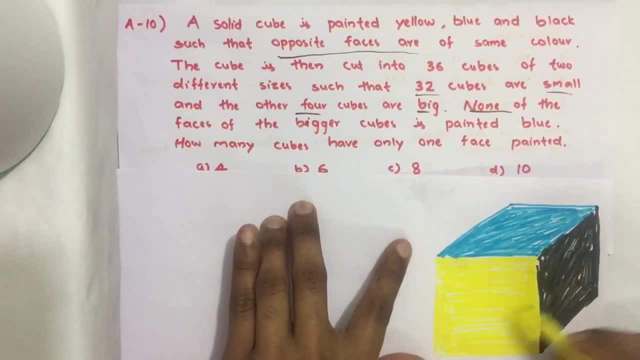 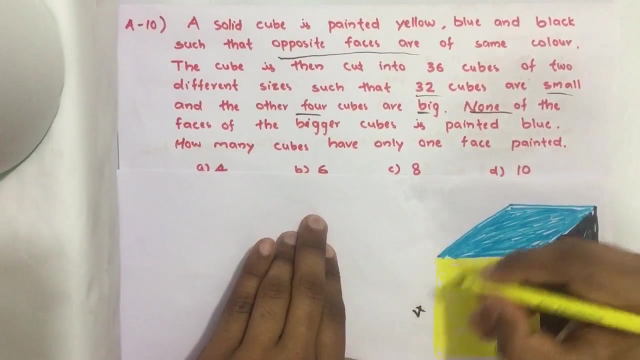 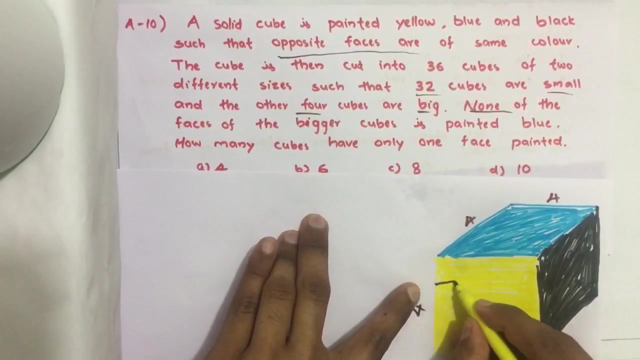 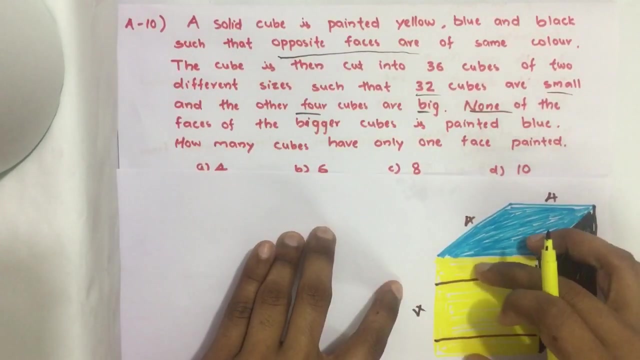 That means the bigger cubes come only in the center side. So we divide this. Suppose it is a 4x4x4.. 4x4x4 cube: We just take the top portion and bottom portion. Here we can only have smaller cubes. 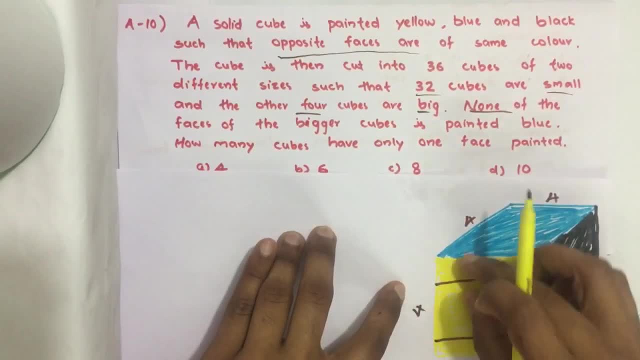 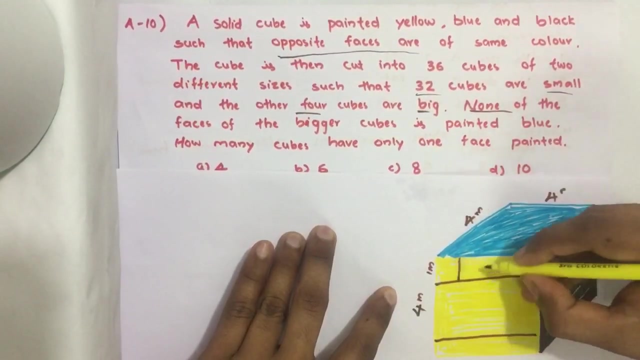 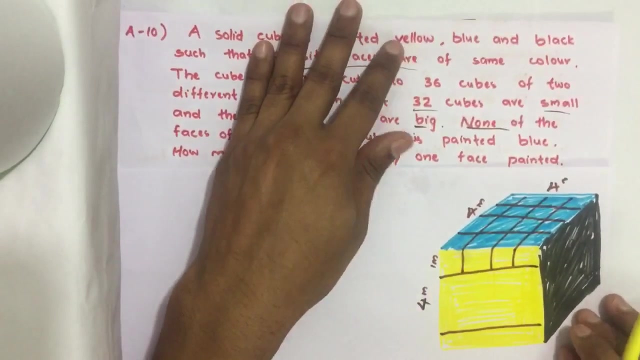 If we are keeping some bigger cube here, that will definitely share the one face in blue color. So if it is a 4x4x4 cube, then I took one meter from here And also divided this into four. You just 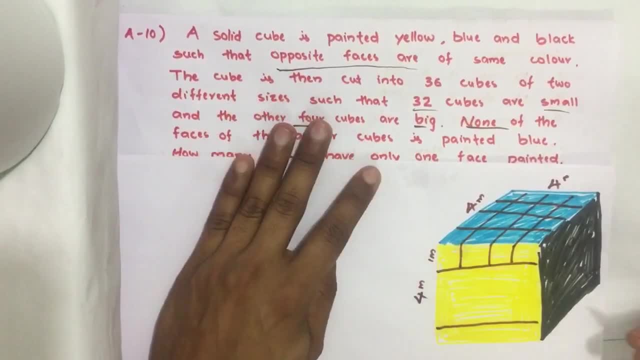 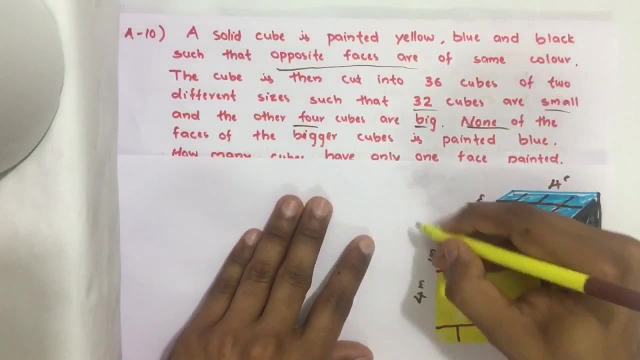 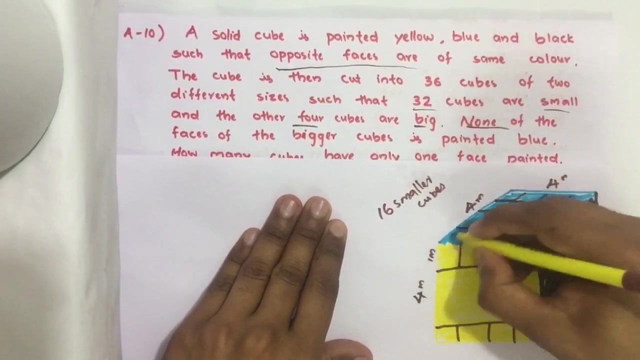 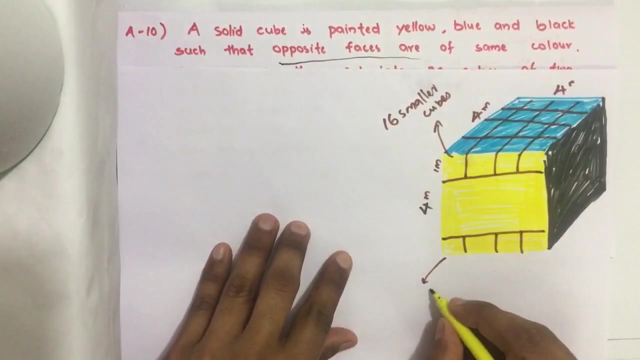 Here we get 16 smaller cubes. Similarly from bottom. Here we get 16 smaller cubes from top. similarly from bottom, we get 16 smaller cubes. The remaining space it is a 4 x 4 x 2, it is a rectangular block.